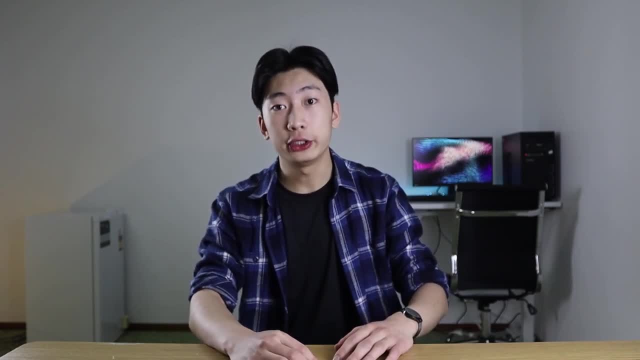 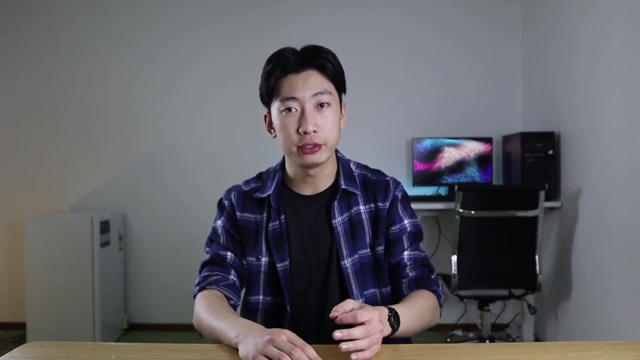 class notes beforehand, And the main reason for this is that research has shown that pre-learning allows you to build deeper connections and therefore understanding, because you've already been exposed to the content and now you're just reinforcing what you've learnt And the analogy that I just 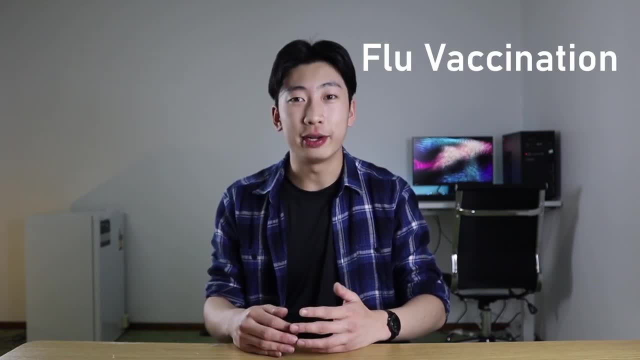 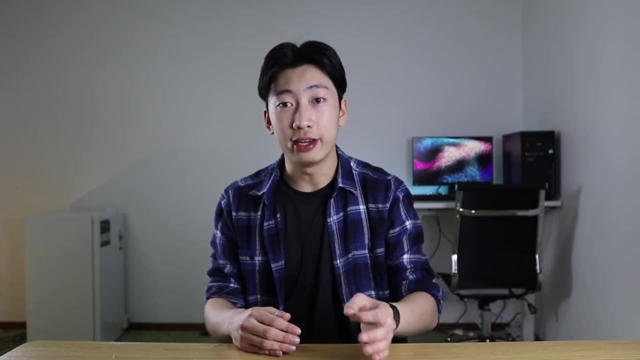 thought of was it's kind of like getting a flu vaccination, because vaccines essentially expose you to some form of the virus so that if you do get the actual infection, your body will be better equipped to combat that. So it's kind of like how pre-learning better equips you for learning the 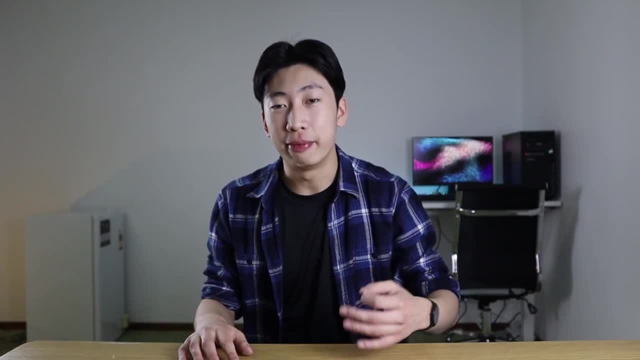 case. So I'm going to talk a little bit about pre-learning and then I'm going to talk about content in class. And yes, I guess that could mean that learning the content beforehand is like getting vaccinated for the chemistry virus, And just to clarify this doesn't have to be long. 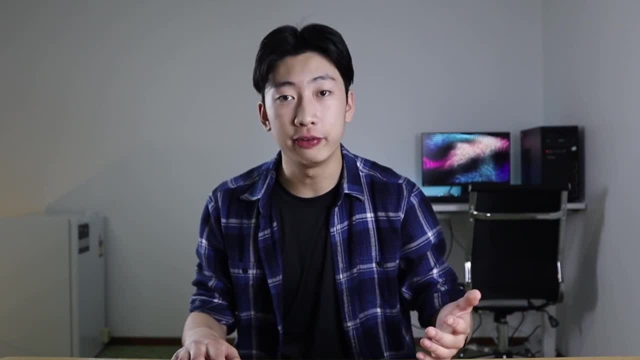 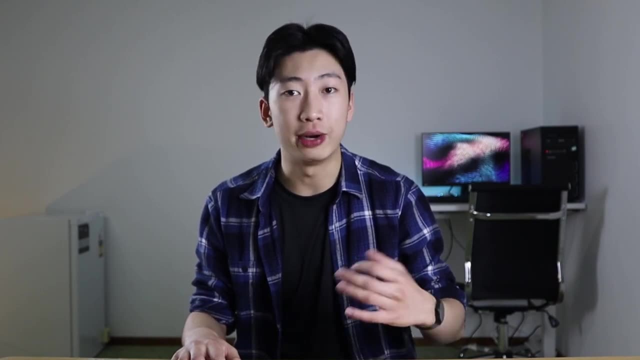 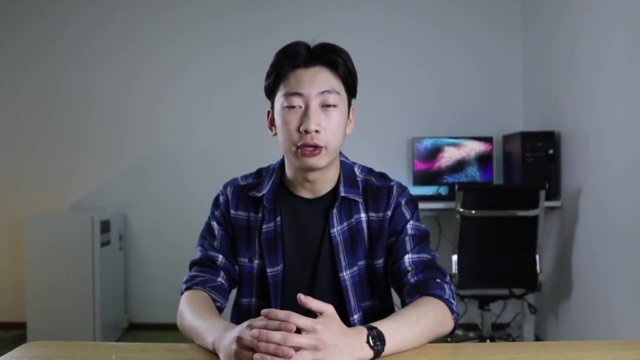 My personal preference was just to watch a short, five to ten minute- YouTube video, and I found that this better helps me visually understand some of the concepts, as opposed to just reading a textbook. And speaking of textbooks, here is how I used mine First, in terms of going through the content. if I'm struggling with a particular area of the content, I'm going to look at the content. If I'm struggling with a particular area of the content, I'm going to look at the content. If I'm struggling with a particular area of the content, I'm going to look at the content. If I'm struggling with a particular. 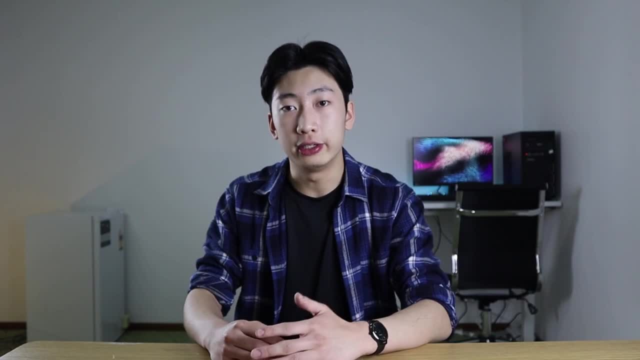 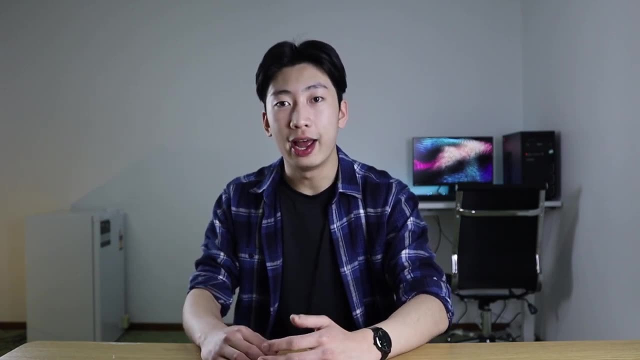 area. I find that looking at the textbook gives a good alternative perspective, But for the most part I use the textbook for the review questions which you can just find at the end of each topic, And even though these aren't like the best design questions in the world, they do help solidify some. 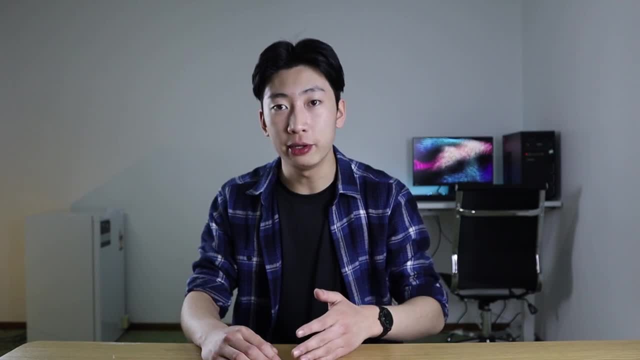 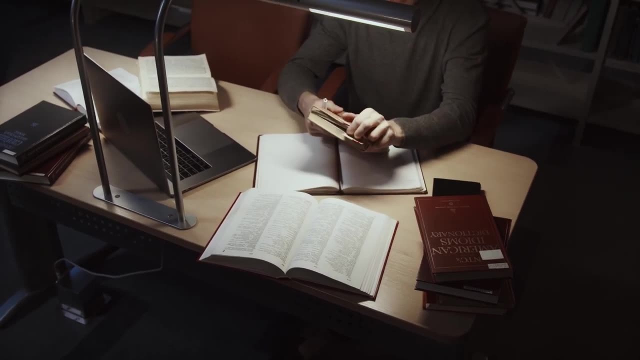 concepts. So this is helpful when you're initially learning something and you just want to check your understanding by doing some simple textbook questions. And of course, you don't have to do all the questions. I just pick and choose until I'm fairly confident with whatever I'm learning. 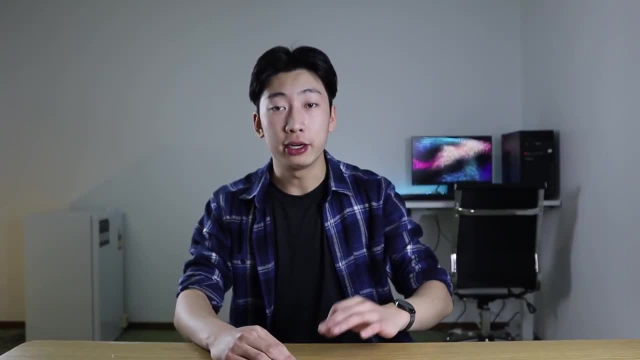 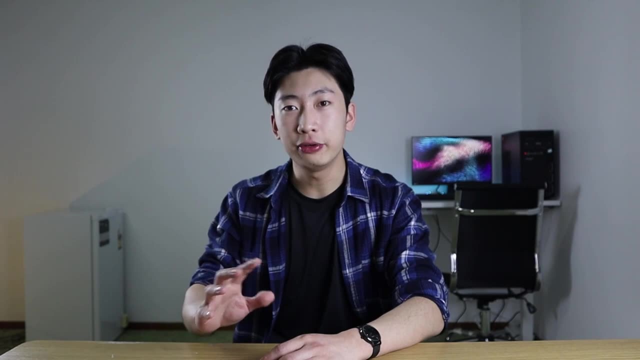 And to make the most out of the textbook questions, I recommend paying close attention to the wording of the answers. So the answers at the very back Now. this is important because this can give you a clue on how assessors are looking for marks, And this is one of the things that many 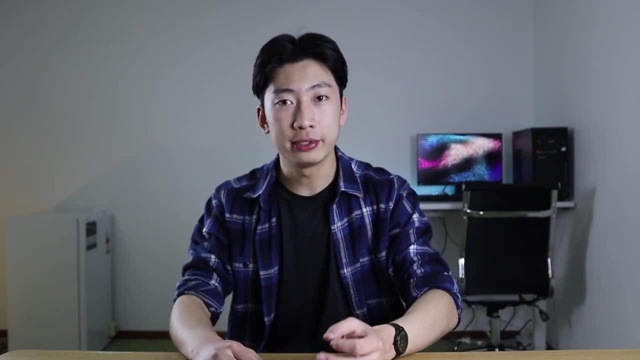 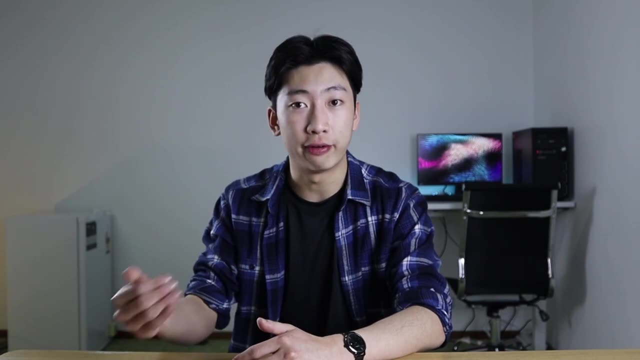 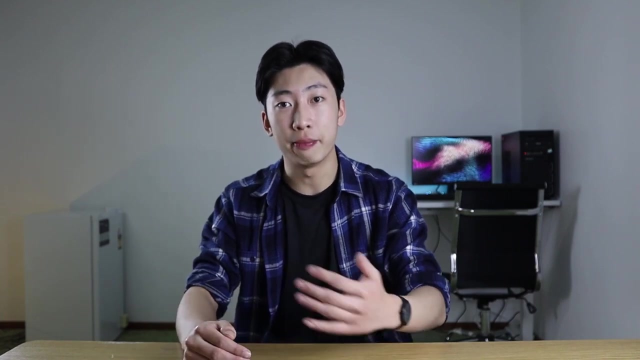 people, including myself, struggle with, Because sometimes you can understand a concept but you might not be able to put that into the words that the assessors are looking for on the final exam. So by looking at the answers after you've done the questions and then seeing if there's any differences and comparing, 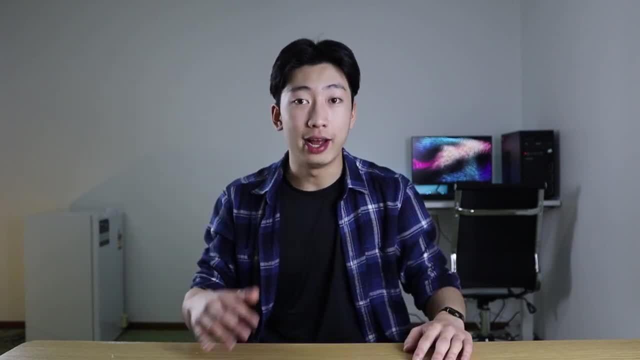 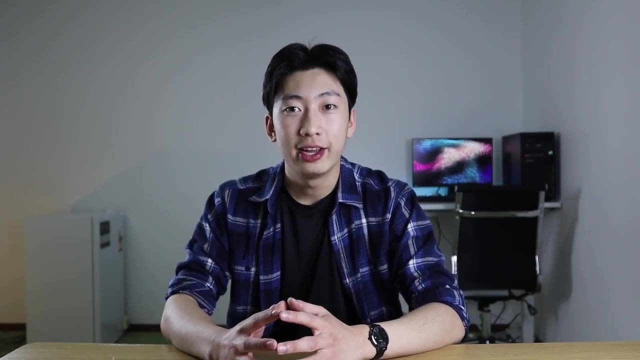 this allows you to be better prepared for the exam-style questions, And this was actually something that I included in my notes, but more on that in a second. Next is note-taking, And I know a lot of people debate over typed versus handwritten notes. 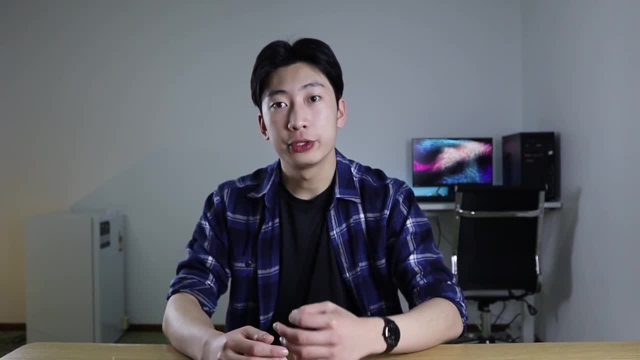 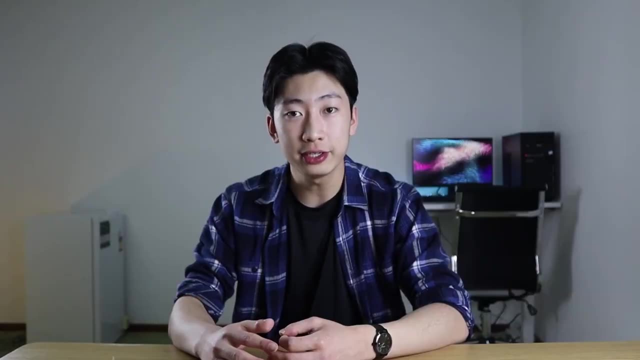 And for me I used a combination of the two. So initially I did my notes on my laptop because it was fast, convenient and I could quickly note down anything the teacher was saying in class, And that way I didn't miss out on important points that were being emphasized. 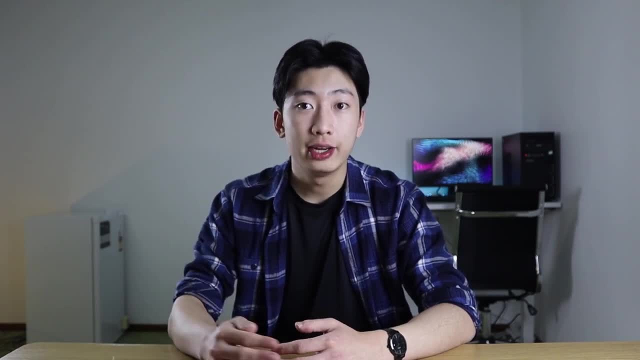 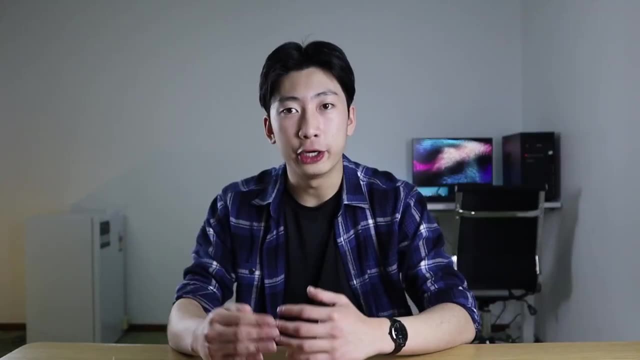 And another advantage is that you can modify your notes, And this is important because you might find that when you watch a video, read a textbook and listen to your teacher, they all talk about a topic from slightly different perspectives. Now, you don't want to have 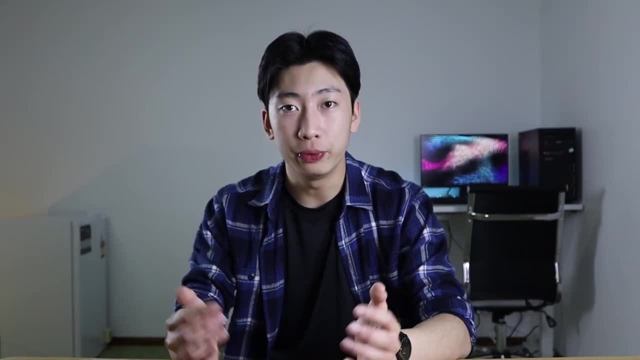 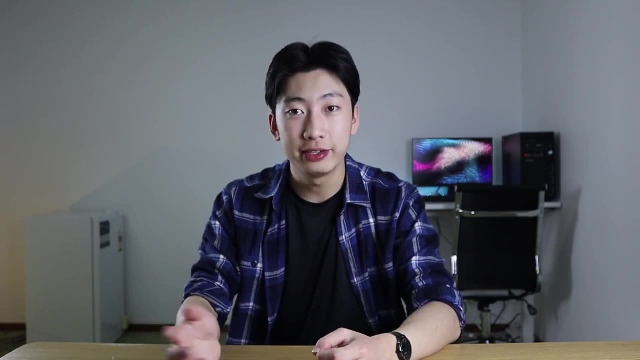 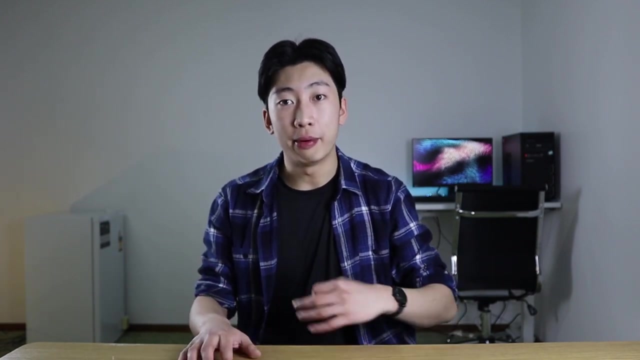 every single perspective in your notes, but instead you want to combine and integrate them into one explanation that makes sense to you, And so from this you can see that I highly recommend, before doing your notes, So after my type notes, feel free to just leave it there. 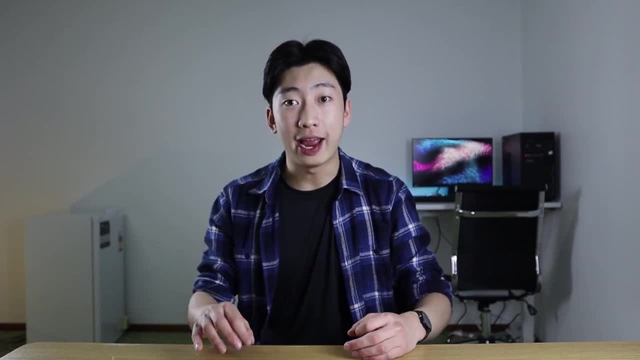 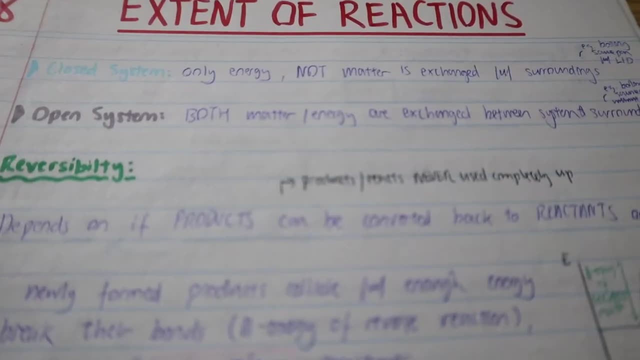 But my personal preference was to practice recalling by handwriting these notes again in a separate notebook and then filling in any gaps if there are. And look, I'm not an arts person, but I did find it helpful to capitalize certain words and add some color here and there. 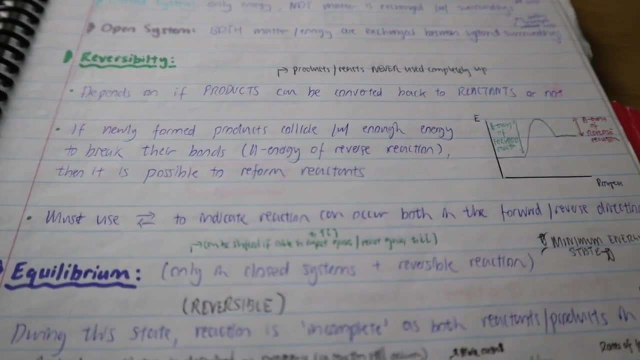 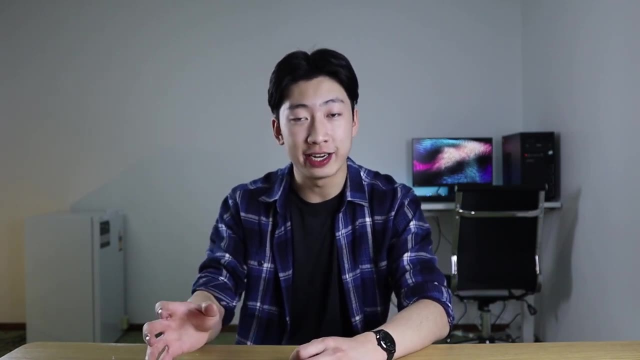 because I found this visually easier to read and also made me want to look at my notes more. So this was my hybrid approach to note taking, which allowed me to exploit the advantages of both techniques. And you might be asking: doesn't this take a lot of time? 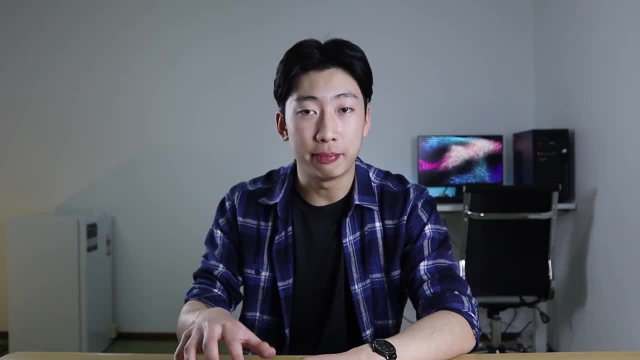 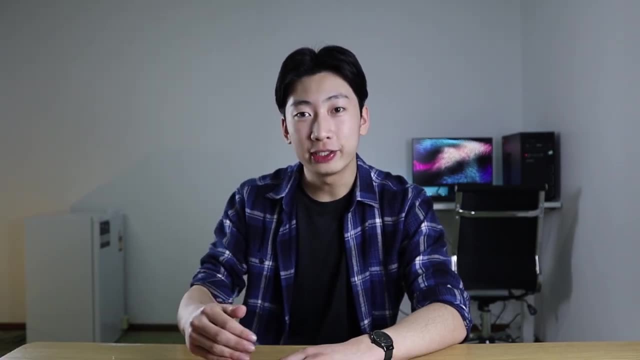 And the short answer is definitely yes, But I found that the more time I spent on making high quality notes- so I'm talking about the quality of the content, not the color or the design- the more time I spent doing that, the less time I spent revising. 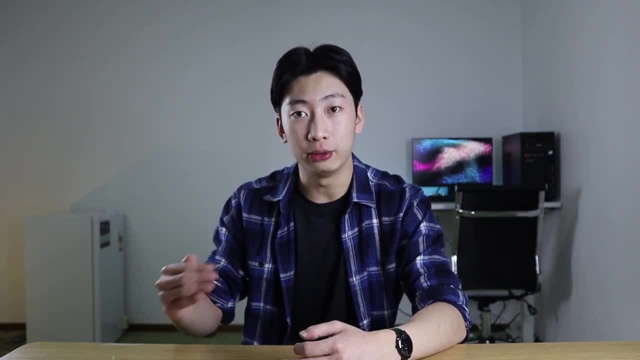 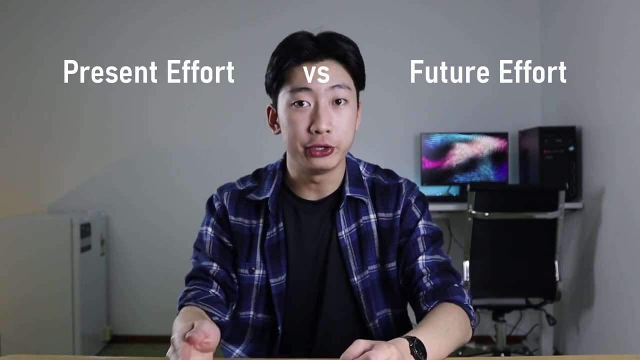 because I understood the content well from this double-layered note taking approach. So there's always a trade-off between how much effort you put into your notes in the present versus how much you need to revise in the future. So we've probably all heard. 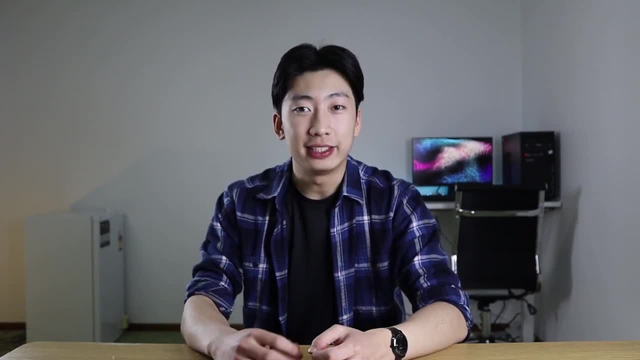 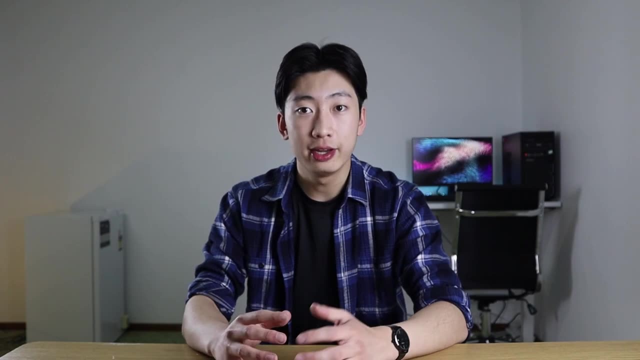 that understanding is always better than memorizing, And it's definitely the case here. And apart from watching videos or other sources, which can help you understand a topic from different angles, another way that can help your understanding is to make your notes more visual. 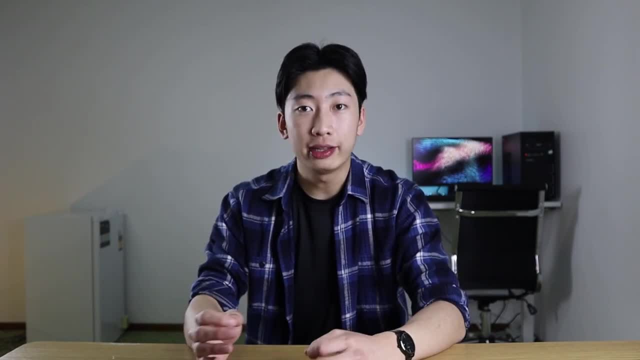 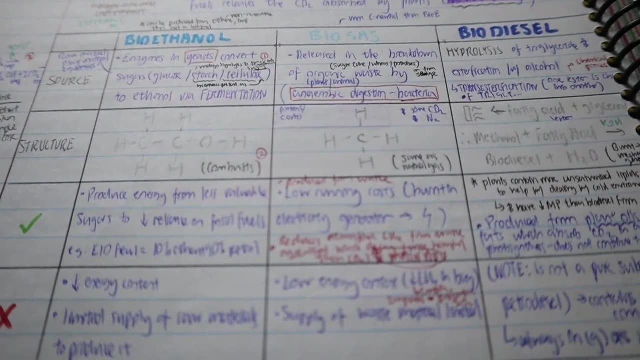 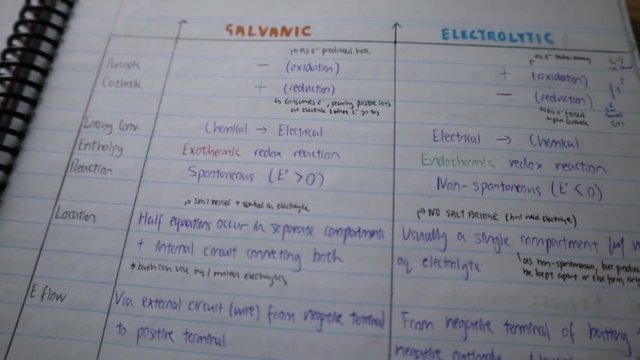 And what I mean by this isn't necessarily adding more color, but rather turning words into diagrams or tables or mind maps. So, for example, tables was something that I used the most when you're comparing two or more things like types of fields, differences between galvanic and electrolytic cells. 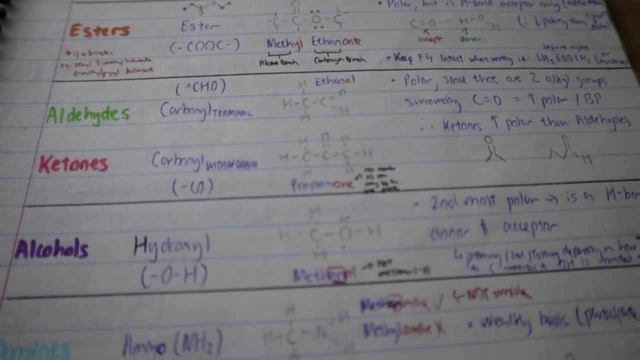 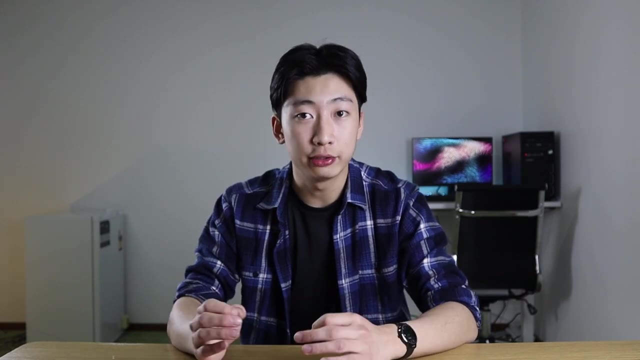 or all the organic cam functional groups. By laying out these concepts in a visual way, when it's usually quite scattered in a textbook, it makes it much easier to see the links between different topics and therefore aid in your understanding. So, after learning, a new piece of content. 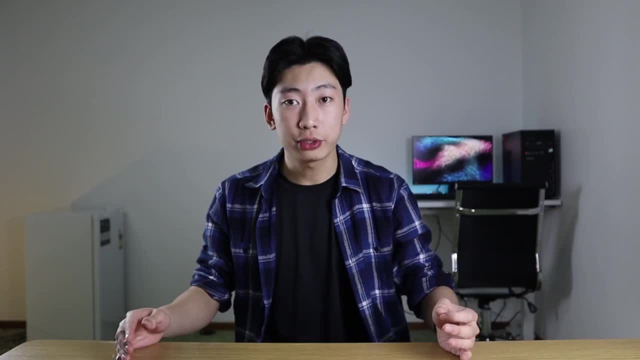 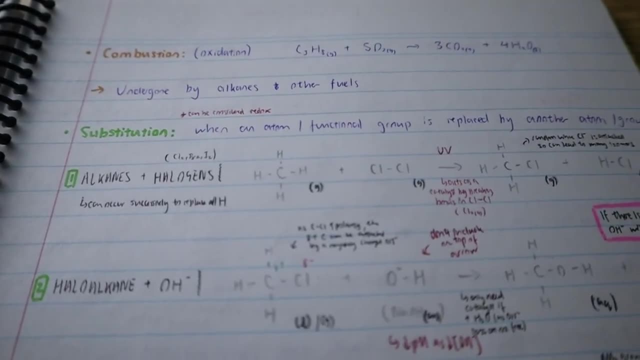 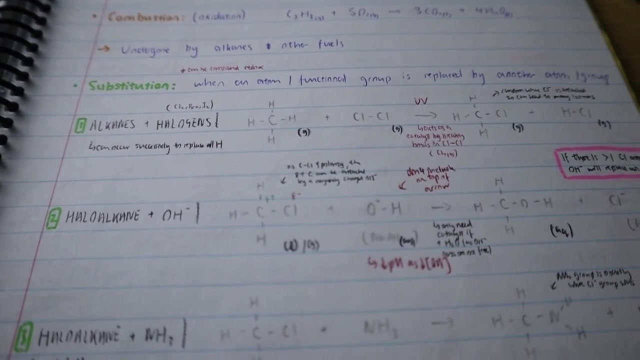 between that and the exam, my process was just doing practice questions and adding anything I found helpful into my notes. So here's what I mean. So your notes are not static. I would always go back and add additional details as I did more practice questions and exams. 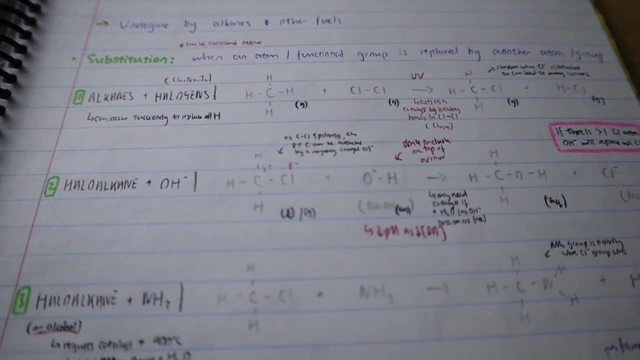 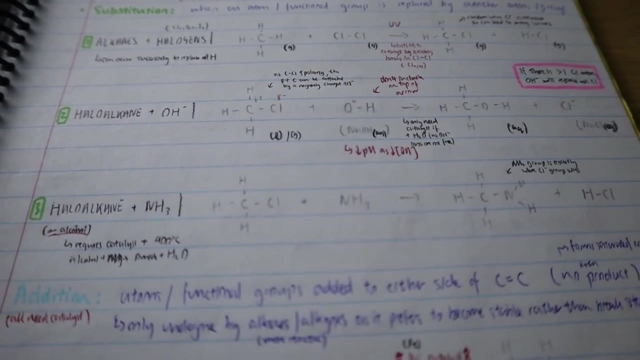 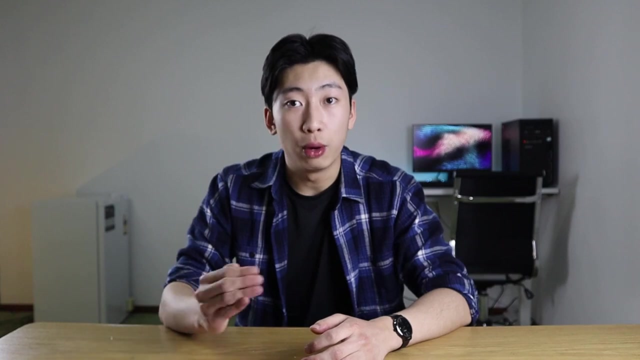 So you can see here in these small black writing, these are all the additional notes that I added after doing more questions, And these basically contained the ways that assesses worded particular concepts, And this is because one of the most important things and important tips is knowing how the assesses. 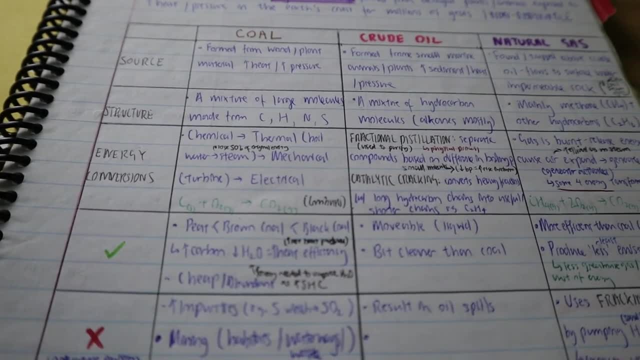 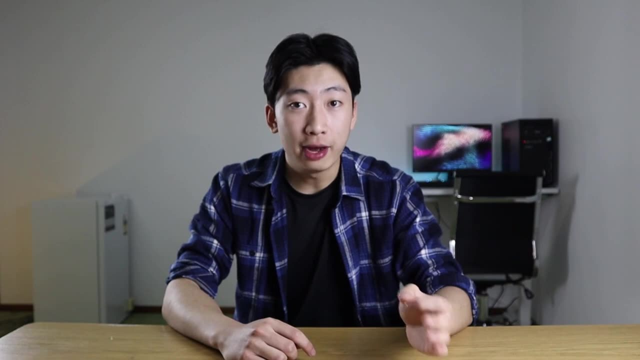 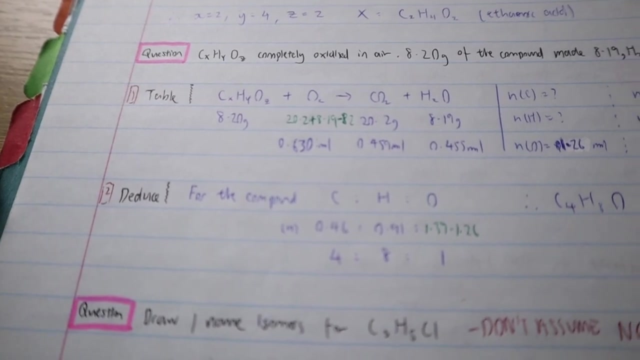 are wording the answers, Because the wording in textbook answers or examiner reports contain particular phrases that maximize your chance of getting the correct mark. And, apart from this, another thing that I added were questions that I either found hard or got wrong, And you can also see that I came up with a set. 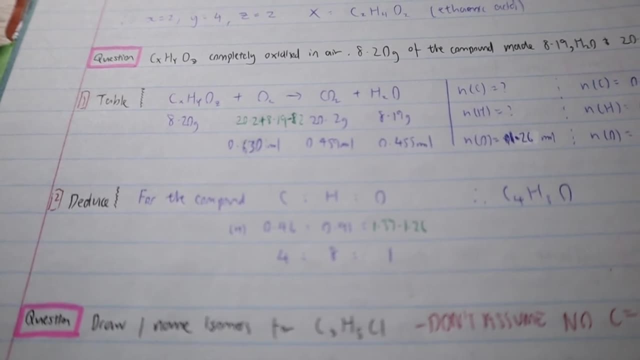 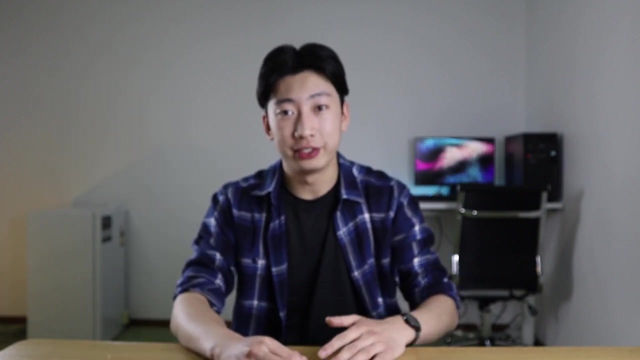 of work solutions for each of these questions, And for me, this was the most important part of my notes, because the final exam is essentially just a bunch of questions. Yep, I know big surprise, But the idea here is that by 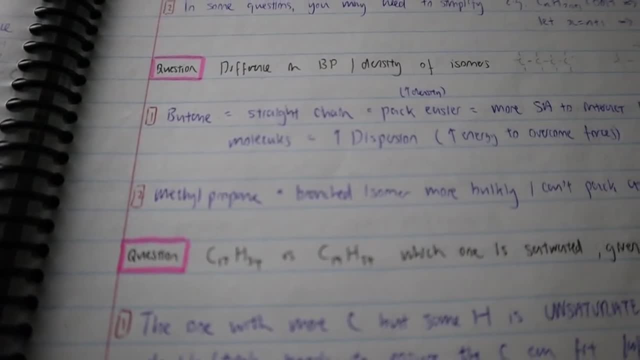 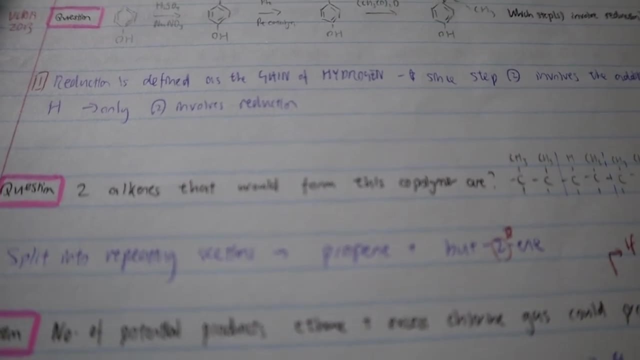 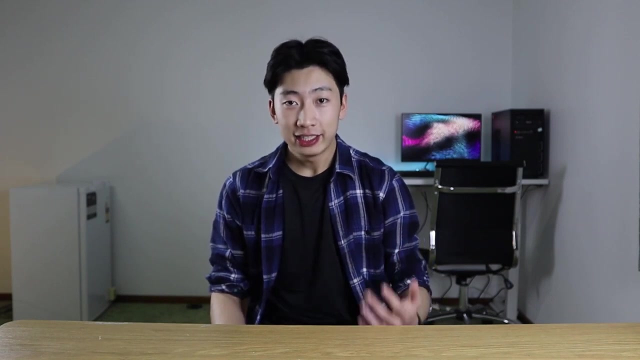 framing your notes in the form of questions. this allows you to first get used to the difficult questions you might see or got wrong, but second, it also gives you a structure for answering these questions. So how often did I revise or review over my notes? And to answer this first, I'm going. 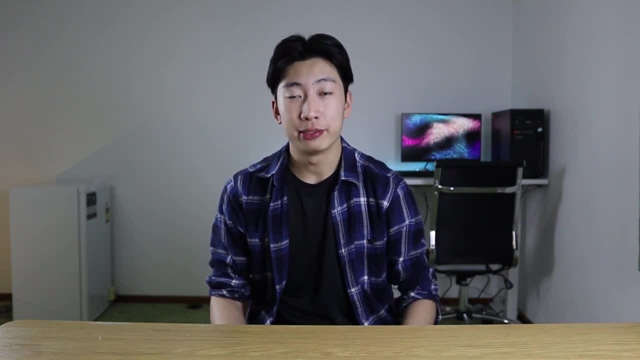 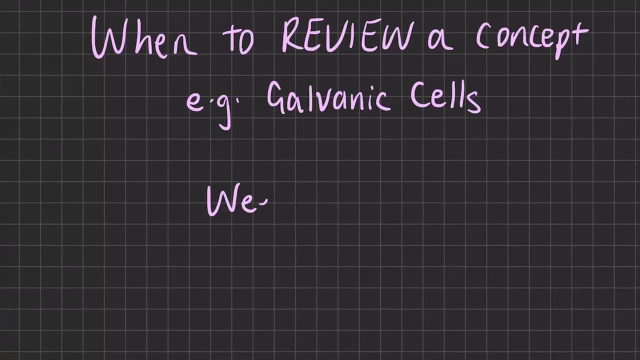 to introduce something called spaced repetition- and you might have heard this before- And this basically means reviewing a concept over increasingly longer time intervals. So, for example, you might review topic one after one week and then look at it again after two weeks, and then again. 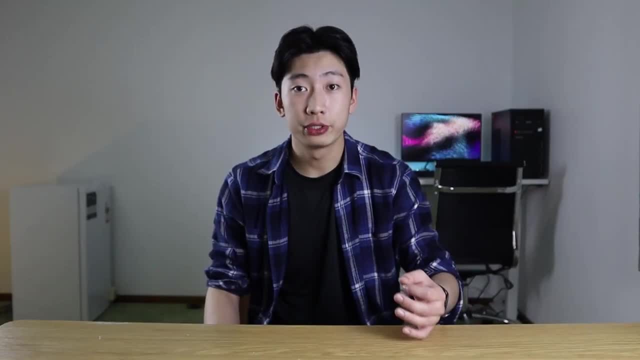 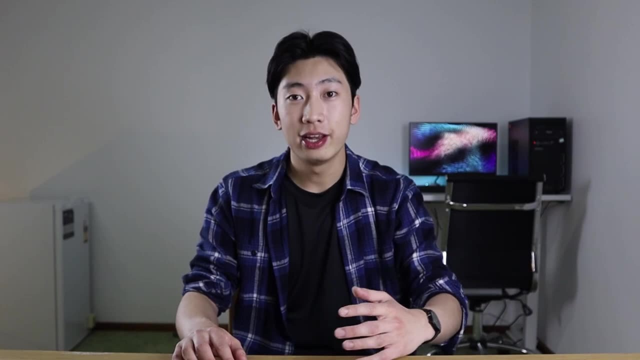 maybe after five weeks, And research has shown that this boosts long-term retention. But I'm not gonna lie. I wasn't disciplined enough to review my notes like every week or every two weeks, so here's what I did instead, So hopefully. first you have a set of detailed notes containing 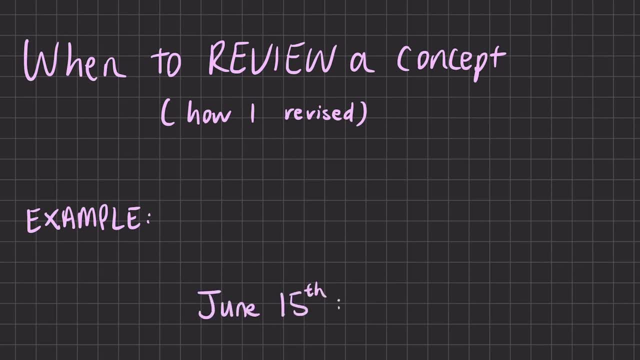 content, questions and also answers. And what I would do was I would just review my notes one to two weeks before a small test or quiz, and a bit longer if it was a sec, And this acts like a quick refresher. And yes, I know this is a bit of a passive process: just looking over your notes, but this is why I 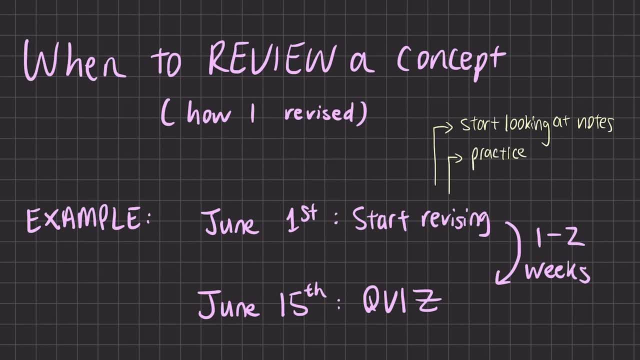 follow this up by doing more questions and more practice sacks and then adding anything new from those practice questions back into my notes. So I'm continually building this resource And then, two to three months before I review my notes, I would review my notes one to two weeks before a 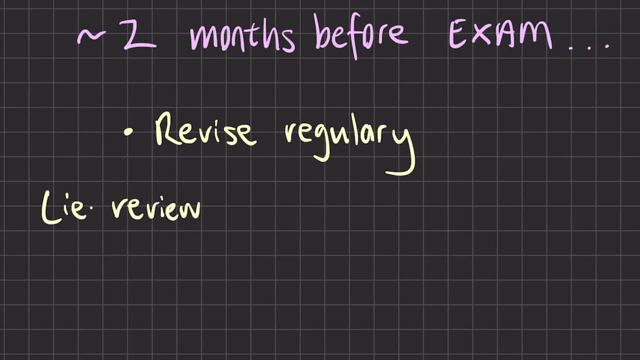 test. I'd review my notes more often and if there's a lot of questions that I have a way to solve, I'd review my notes over the next three or four weeks before the final exam, and that would be the same, And then the results would be similar. like I said, I would review my notes more regularly. 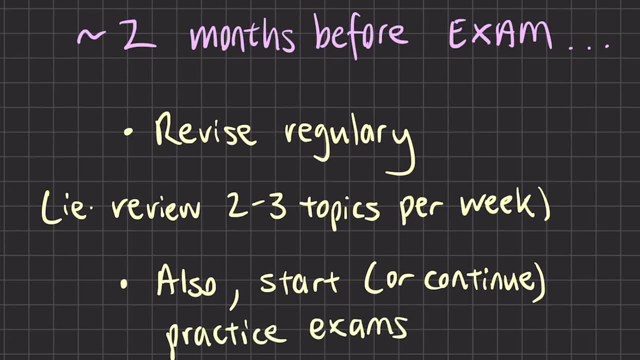 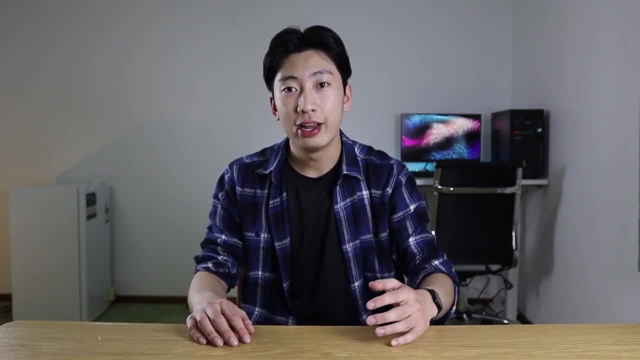 so in a more spaced repetition kind of way, And that was just because the exam is obviously much bigger and there's much more to remember in that case. So I'm not saying that this technique is going to work for everyone, but it was practical for me And that's why I used it. Also, I wanted to 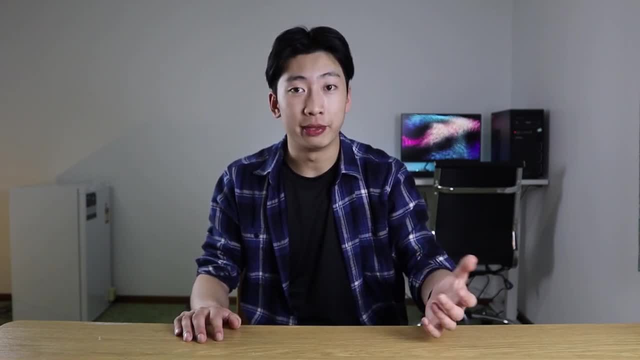 shed light on what exactly I did to get a raw 46 in chem, but feel free to make any adjustments from this, As much as I do understand what you meant by doing your test. I'll probably try it again in the next few weeks. 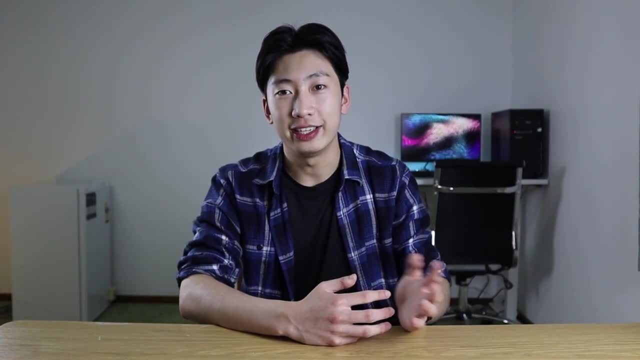 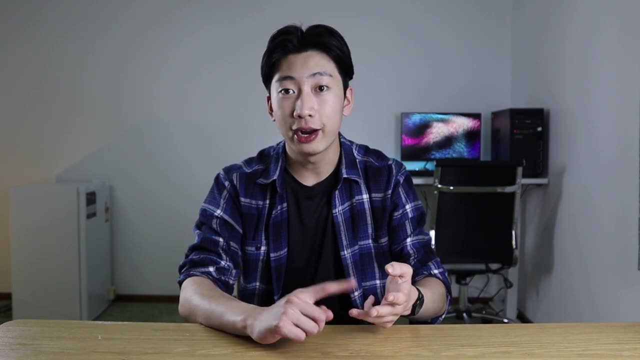 Um, as much as I hate sig figs, yeah, you gotta know them. And just as a bit of a bonus tip, whenever you're doing notes or questions or practice exams, start using dot points and shorthand, because both of these will save you a lot.